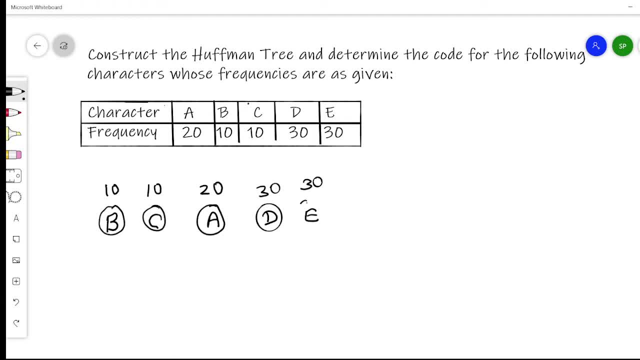 now in sorted manner. What we will be doing is we will be taking two nodes, which is having minimum frequency, and combine it together. So this B and C we will take together because those are the having frequencies- 10- and those are the minimum frequency. So 10 and 10,. 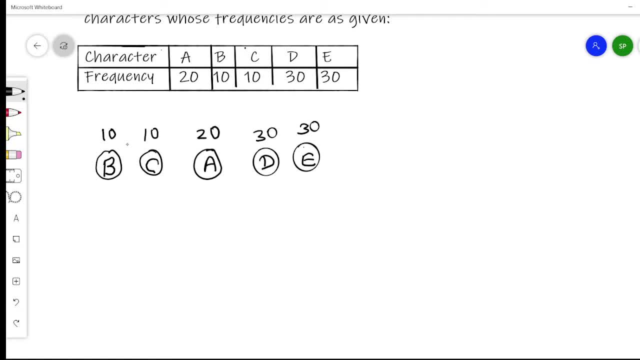 we will take and combine it together by taking the sum of this one. So 10 plus 10 is 20.. So we will be getting 20. and then what we do? we will be having the children as B and C. We have the. 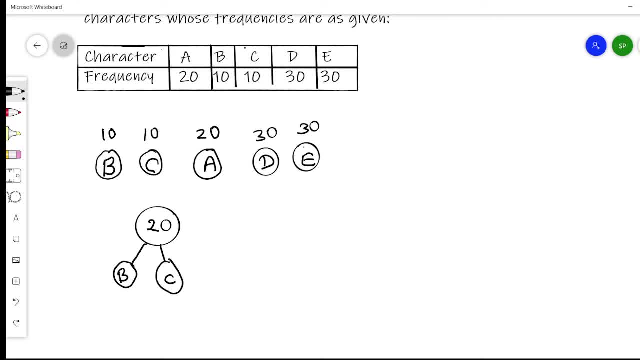 children B and C. Next one, when you see this one. okay, I will just take down that one and write it here: We have 20, we have 30 and we have 30. This 20 is corresponding to A, this is D and this is. 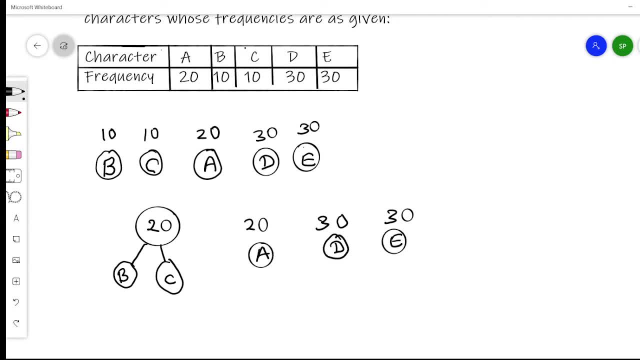 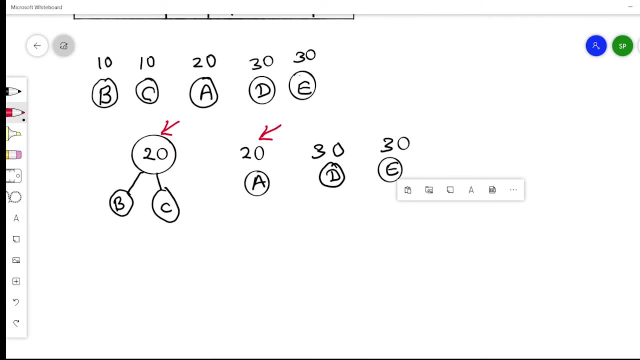 B. okay, So this one. now we have to take the minimum from this. So we know that this 20 is minimum and this one is minimum, This 30, both are more than this 20.. So minimum two will be this, the first 220 here. So what we have to do is we have to merge these two nodes and form a single. 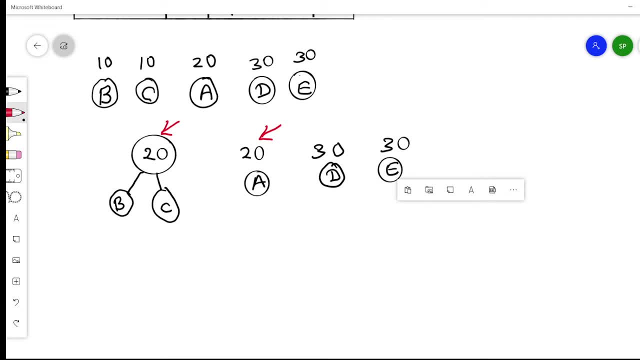 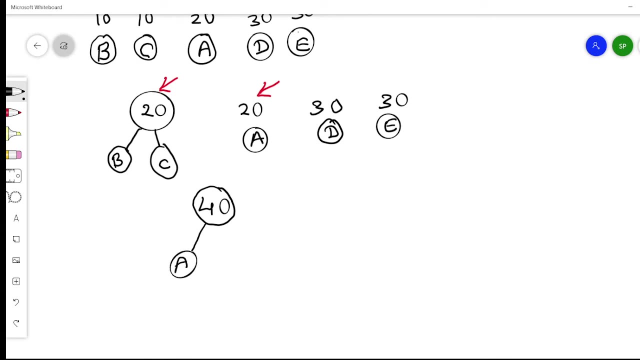 new node, that is, by taking the sum of the values of this one, that is, 20 plus 20.. We will be getting, and the left child will be taking it as A. okay and right, we will be taking this one here, this 20, and B and C. So that is our this one. I will just: this is B and C. Now we have. next we should see what. 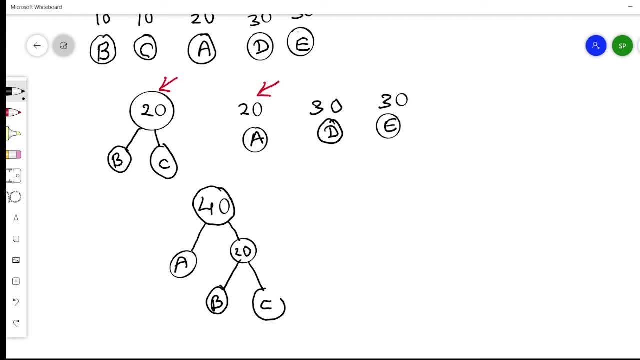 are the values present, The next two minimum values we need to see here: 40.. Now we have taken, we have taken this node. we have taken this node. Now, what is remaining? this? 30 and 30. okay, So here we have this: 30 and. 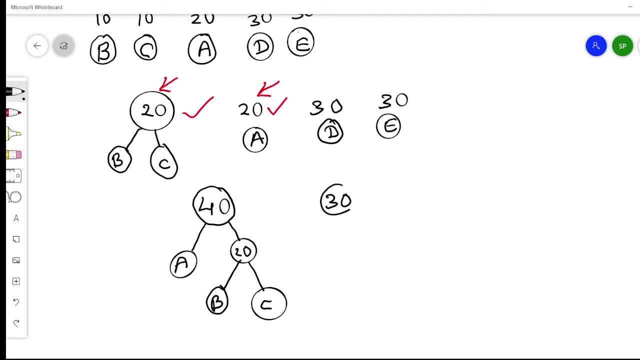 30. Let me write this here: 30, and this one is 30. okay, This is D and this is E. okay, Now the next two minimum values we need to take. So one minimum value is this: 30. The second minimum value is this: 30. So we have to combine this two and form the new node. So 30 plus 30, we will be. 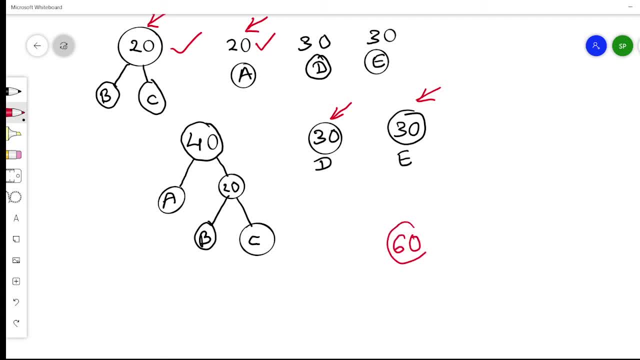 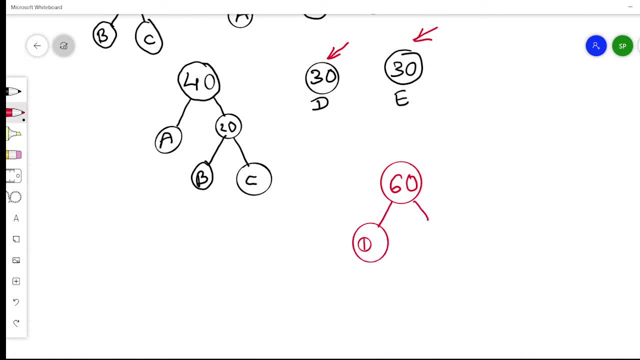 making it as 60. okay, I will be getting it as 60. Then the node values will be D and E. here And on left side, we have this 40. okay, We have this 40. Then A: the same thing I am just writing. 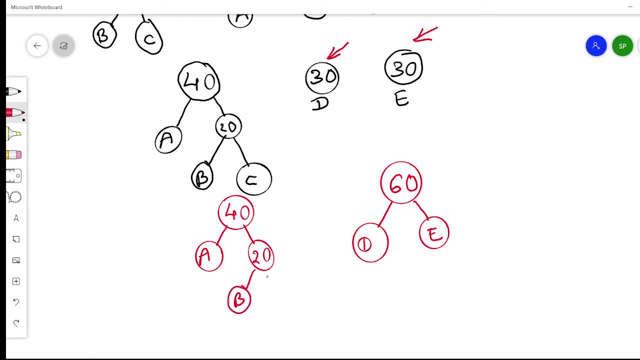 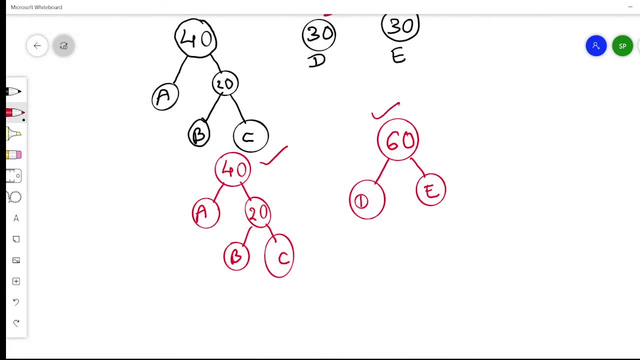 it again: B, C, okay. So this we have, this two now, 40 and 60 we have. So we have to combine this. two form the new node. So 100, we will be having 100. So 100 is our new value. Then on left side we have: 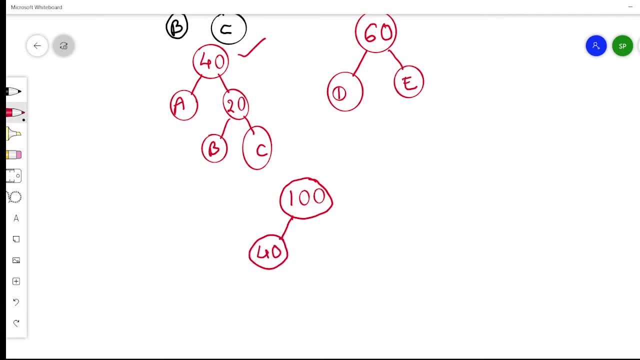 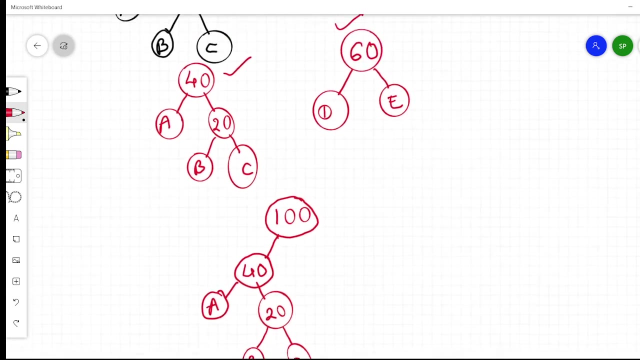 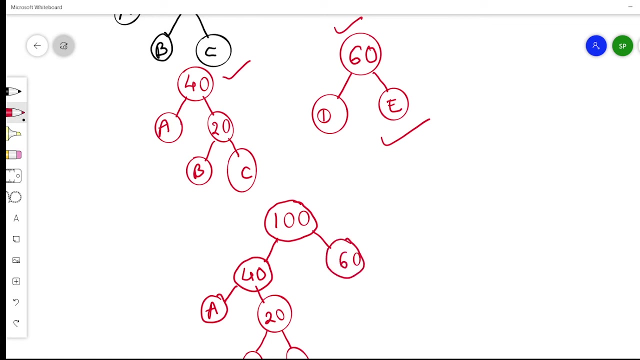 this 40. And then A, We have this 20, and then we have B, and then we have C on right side And 100. on right side we have this, the whole thing, this one, that is 60. The node is 60. And on left side we have D. 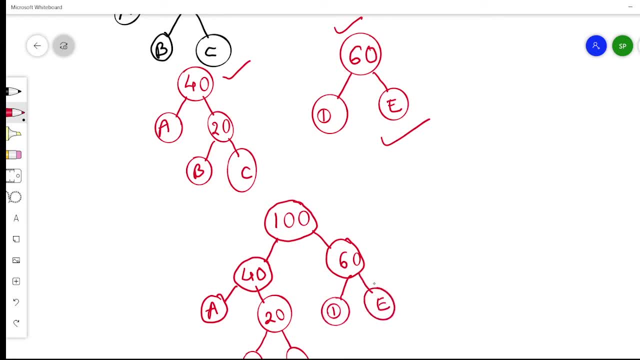 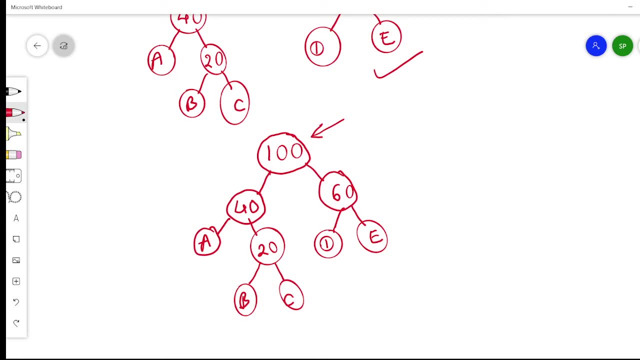 and on right side we have E. okay, So now, if you see we, we are left with only one node here. So this is the final Huffman tree, okay, So we have to do this process till we reach the single node as a root node. So this one, the tree which we got here, this is our Huffman's tree. 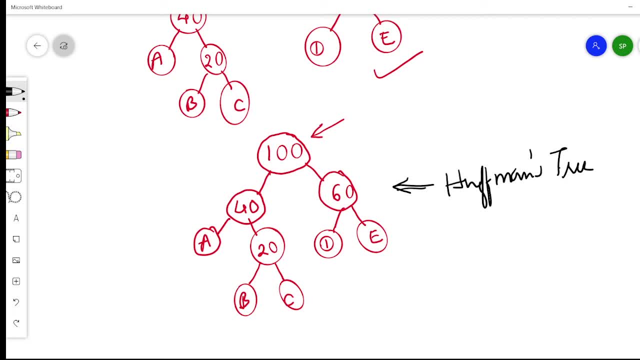 Huffman's tree. Now how will you find the code? okay, So for finding the code of this characters, what we have to do is, on the left side we have to assign value zeros, And on right side branch we have to keep one. So this is right one. 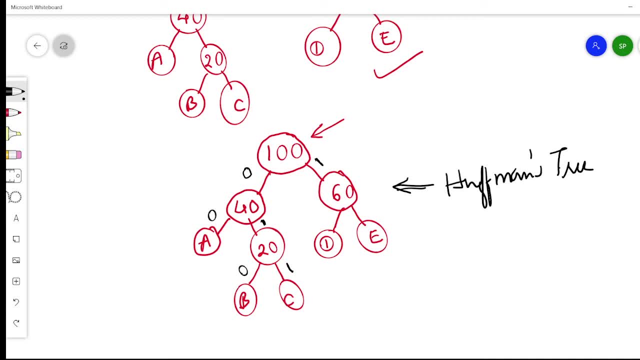 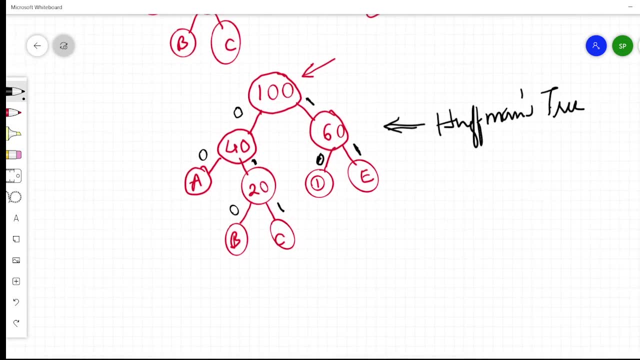 Here left side we have to keep zero, Right side it should be one, And here left side it should be zero, Right side it should be one. okay, So now we have just put the codes here: On left branches we have to assign zero, And on right branches we have to assign one. Now see here all these characters. 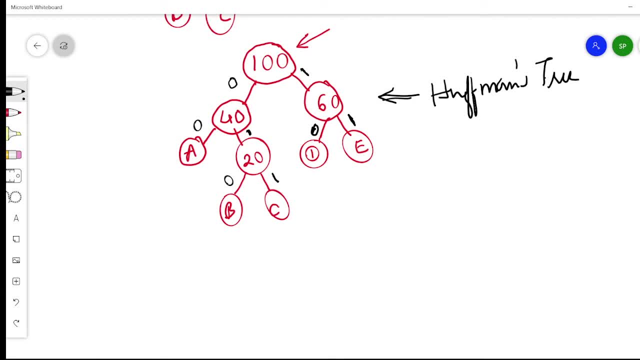 A, B, C, D, E are all present as the leaf nodes. Now if you want to find the node or this code of A, how do you do that? You have to see: start from this root node, go up to this A, So from root node when. 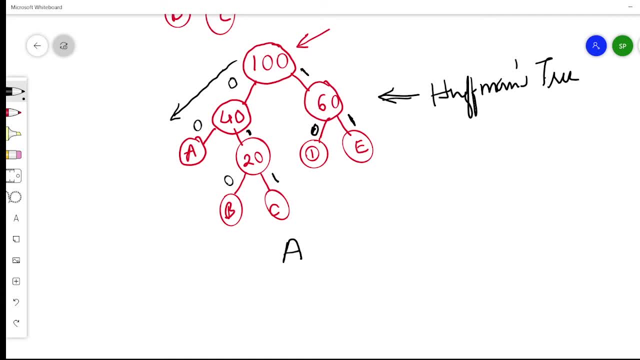 you are traveling up to, traversing up to A, you are getting zero, zero. So the code is zero, zero. Now B. we talk about B. we start from this root node. we will be starting from zero. We will be starting from zero. then we will be coming like this: right, So zero, then one, then zero. So we will be getting 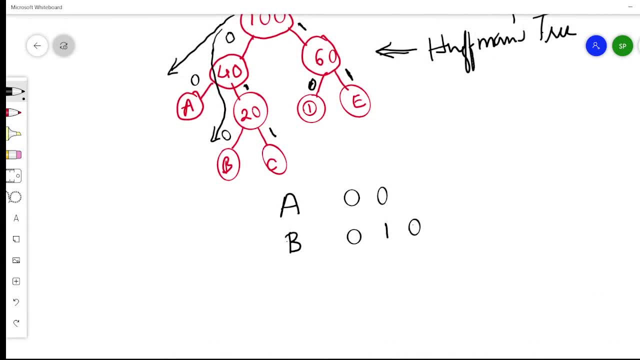 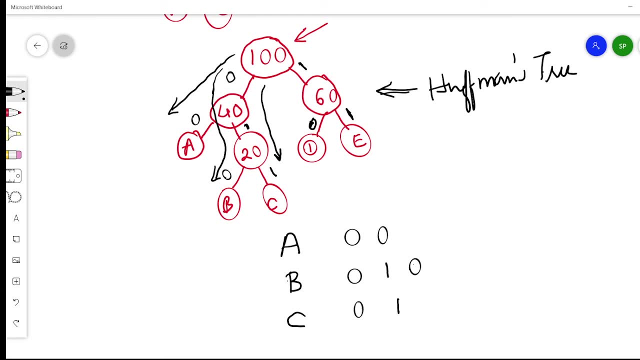 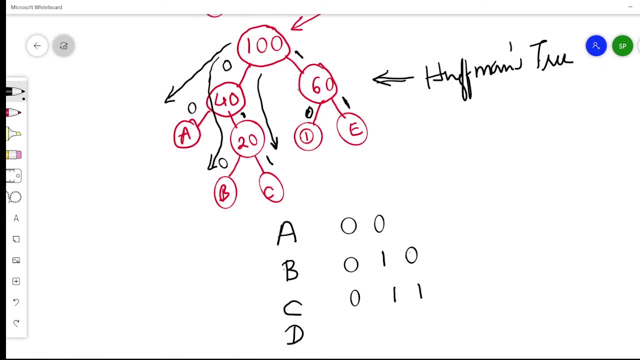 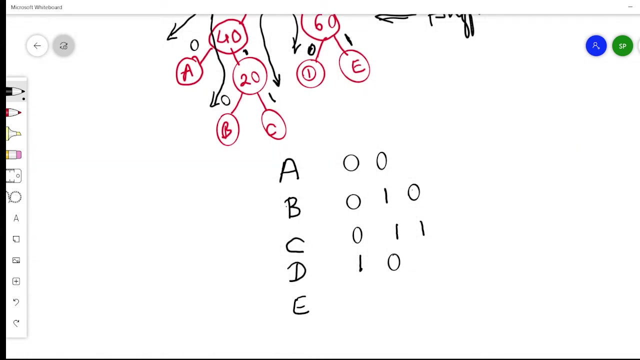 one, okay. And now we have C, C, the code is when we are coming, traveling like this: So it will zero, one one. Now, coming on to D, we will be traveling from the root node. Then D is like this: So one zero, one, zero. And what about E? E, you have. you will be traveling like this: from the root node. 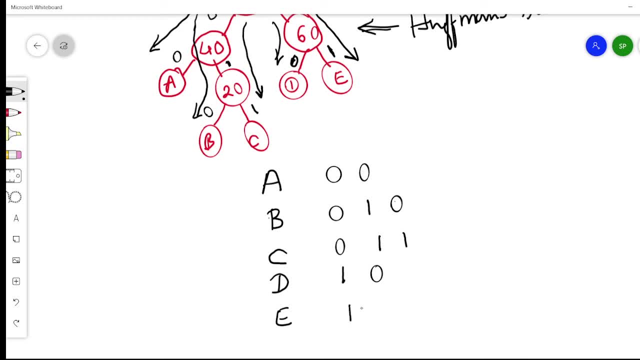 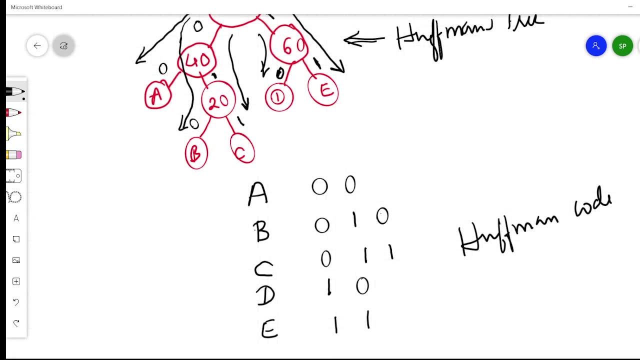 So it is one one, So one one. So this is our Huffman code. Code for the characters. Okay, So you could easily find the codes from this particular tree, Huffman tree. Okay, By assigning the left branches as zero and right branches as one, And when you. 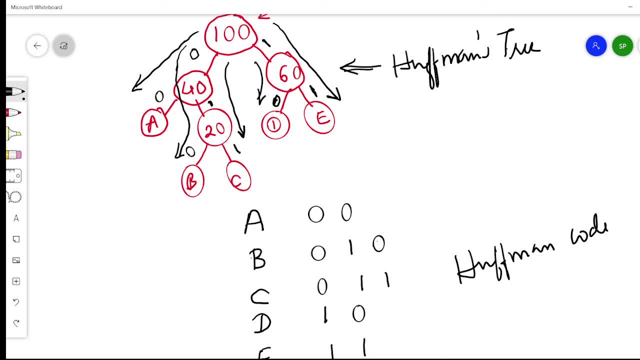 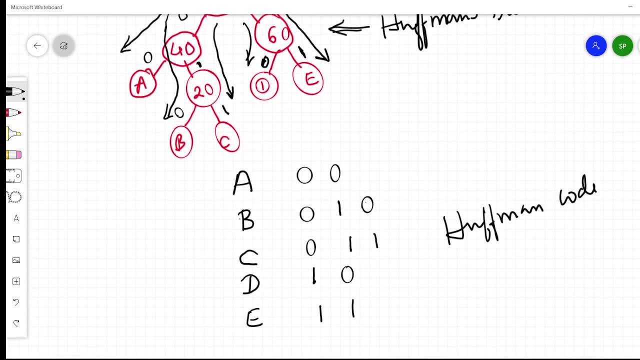 trace back to that particular. when you trace from root node to that particular node, leaf node, you will be getting that code for that particular character. Okay, So this is how you can form the Huffman tree Huffman code. So one more thing you need to remember is that whenever, suppose two values 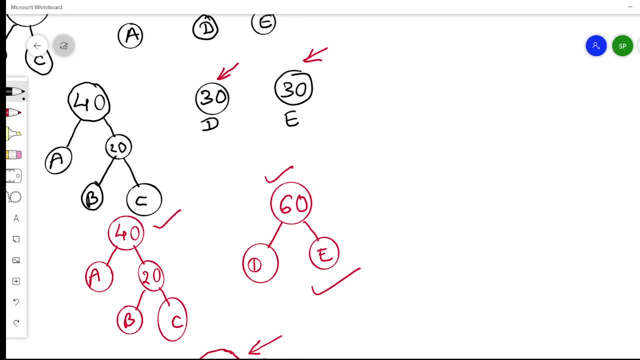 are matching like this, this D and E. So if, if one more is there- suppose I have one more as 30. Then I can choose any one of that and form the tree. But only thing is, you won't be, the tree won't be. 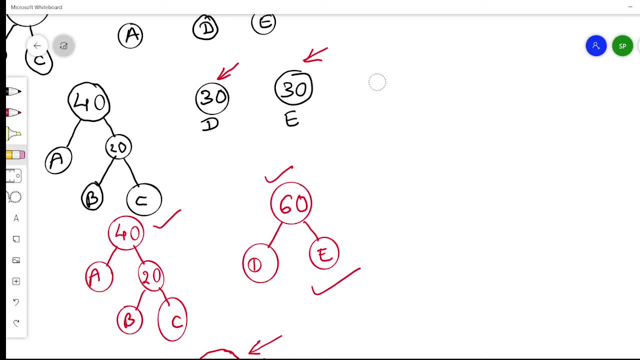 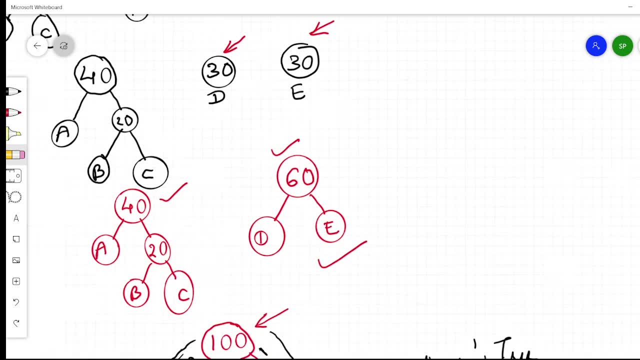 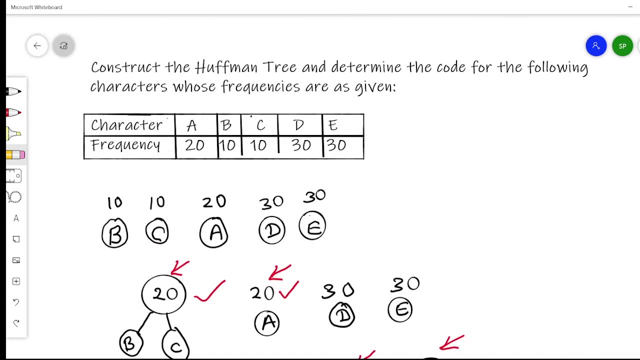 unique. You will be getting a different tree, So the Huffman tree will be different. if you are, depending upon which, which two nodes you are selecting first, the tree branches will be changing. Okay, So this is how you can form a Huffman tree from a given set of values and here, if any, 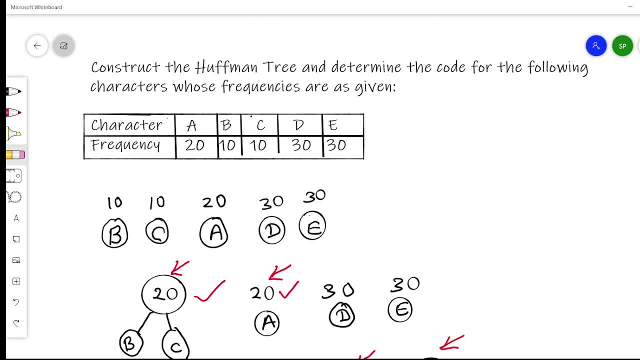 word is given. what you have to do is a particular word is given, You count the number of times a particular, a character or the alphabet is repeated from a table like this and and then arrange it into the sorted manner, and then from the Huffman tree And once you form the Huffman tree from the Huffman.